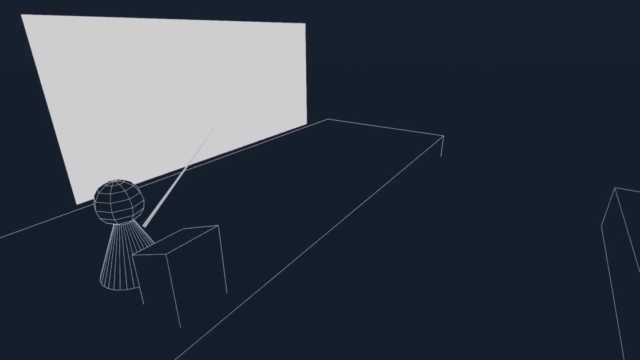 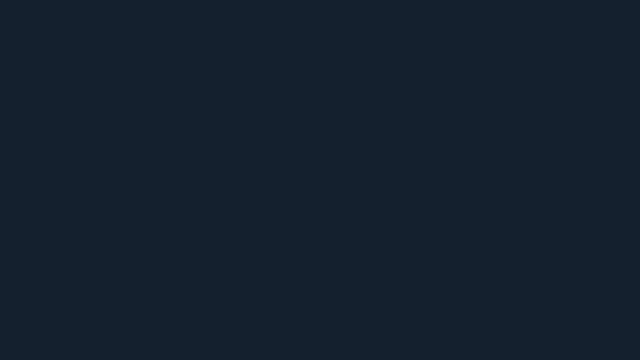 Me and a bunch of my colleagues were struggling a lot with this back then, so I want to give you an introductory lesson on how to prove anything. The subject of a proof is a certain statement, which can be true or false. There are two important types of statements to prove: ones that say something about all objects of some. 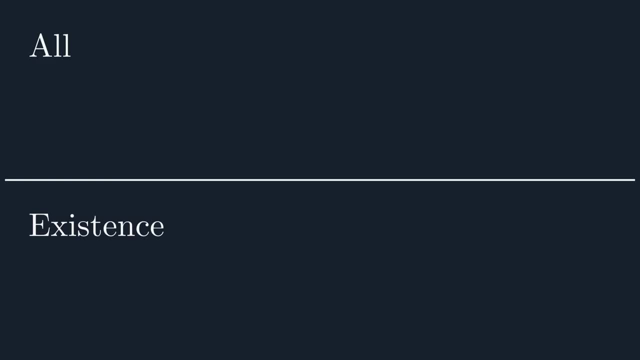 type and the ones that only say something about at least one object of a given type. Here are two examples. All prime numbers are odd. A whole-number smaller than 0 exists. Now, aside from the fact that the first statement is false, we notice that it provides a statement. 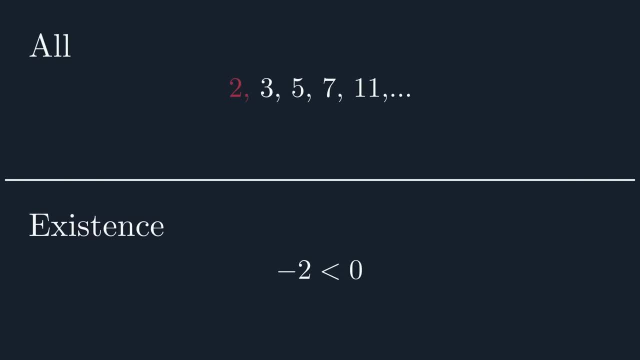 about all elements of a certain type, in this case prime numbers. We denote these kinds of statements with this upside down A here. The second statement, however, gives us some information about at least one element. There might be multiple, but there must always be at least one element of each kind. 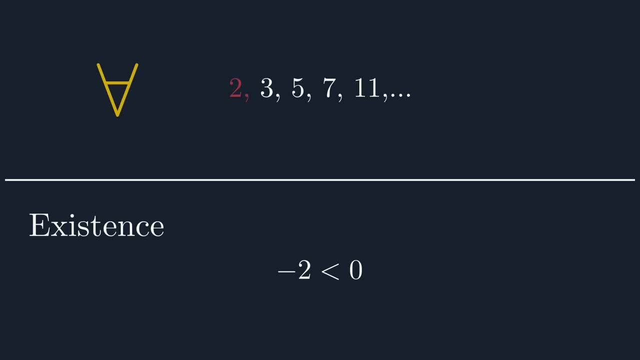 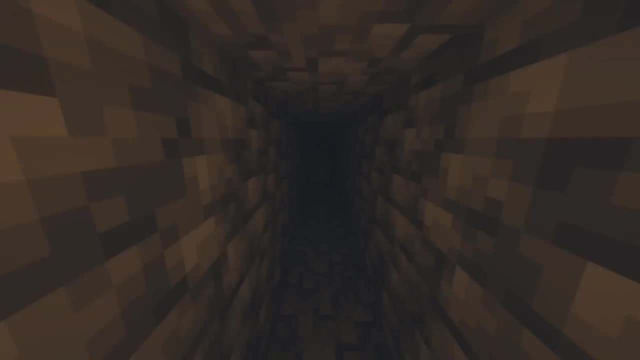 You can keep studying my PhD and your chunk being greater than 3 miters, less than 2 machensitive grams of a constant least one, which is usually denoted by this mirrored E. Now, to create meaningful statements out of these types, we need logical as well as set. 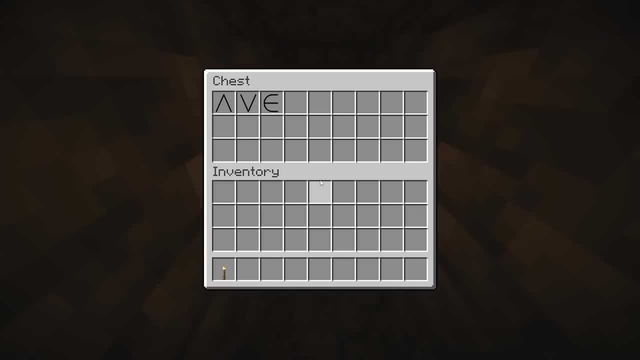 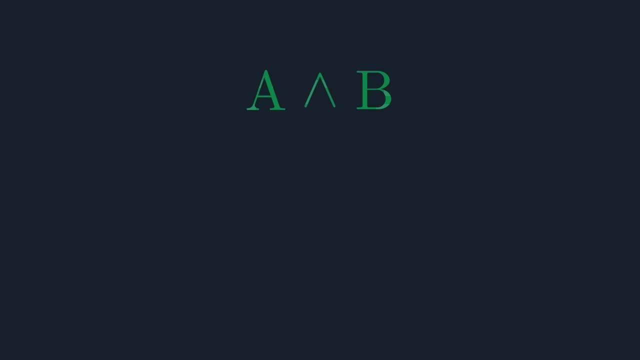 theoretical operators. In our starting inventory we only have three of these. This one is called AND combines two statements and evaluates a true if, and only if both of the statements are true. And the next one is called OR and is quite similar, but evaluates a true if, and only if. 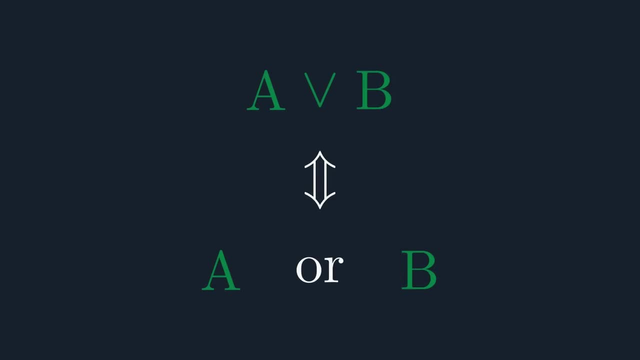 at least one of the statements is true. Why am I putting so much emphasis on the if- and only if, You may ask? Well, that's because you will hear this a lot when doing any kind of research on mathematical topics, and it just means that the relationship described works both ways, as we notice in 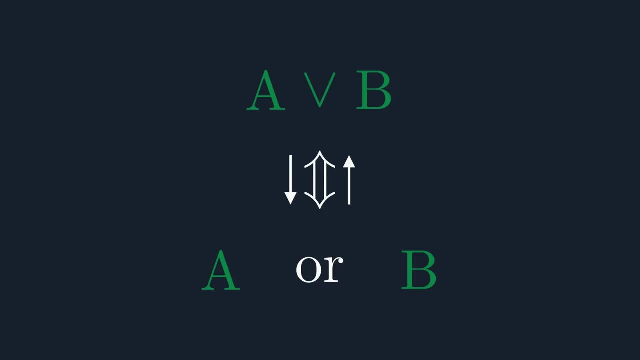 the previous usage of the phrase. If statements a and b are both correct, that would be a positive statement. In other words, if they are both right, then it would also be a positive statement. If statements are both wrong, then it would also be a positive statement. 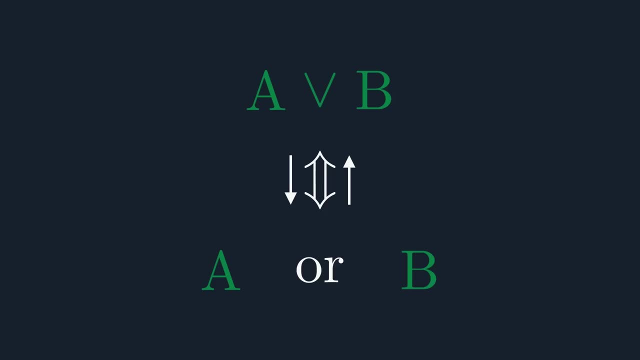 true, then a and b is also true, but this also works the other way around. and to get started, we will also need one set theoretical operator called the in or element of operator. a set is what we just call a collection of things, and we can use this operator to explain the relationship between an element and a. 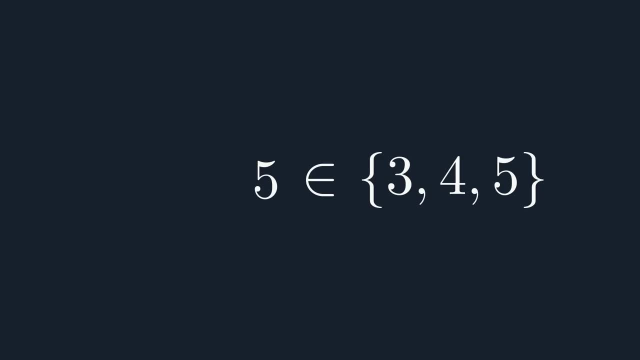 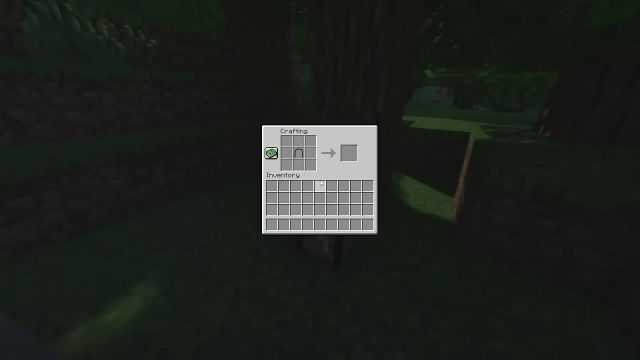 set of certain elements. for example, we could say that the number five is in the set of whole numbers usually denoted by this fancy Z here. with these three operators in our pocket, we could now also go on to define more advanced operators. an intersection, for example, is an operator that's very easy to. 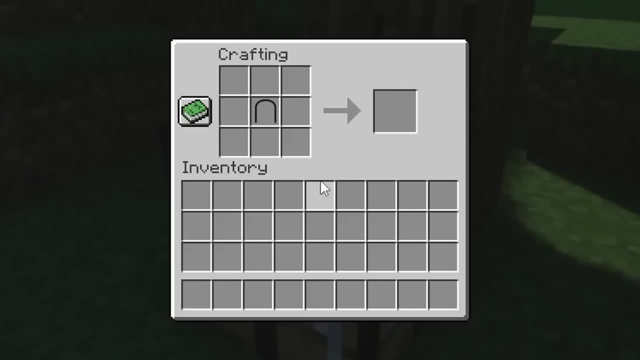 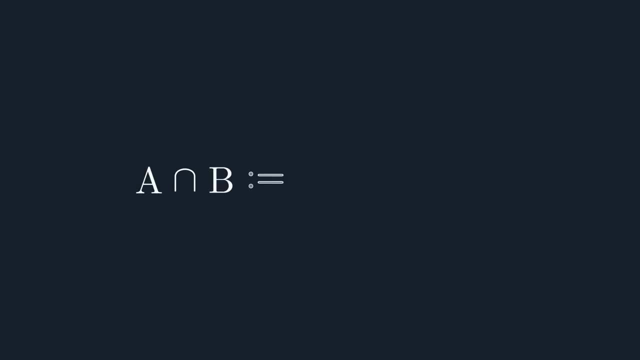 understand visually, but with the tools at our disposal we could formalize it a bit. for example, we could say that the intersection is a set of elements and the set of elements is a set of elements. the section of two sets, a and B, is a set containing only elements X that are 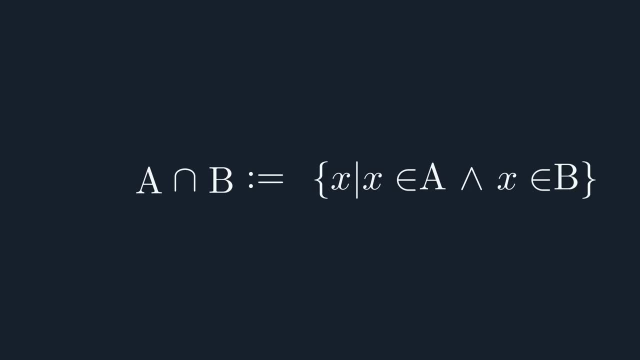 element of a and element of B. you may notice two things about this definition, the first being the structure of everything. the curly braces used to denote a set definition, the declaration of a variable, X here- and the condition section for the X to be included in our set. the second thing is the abundance of 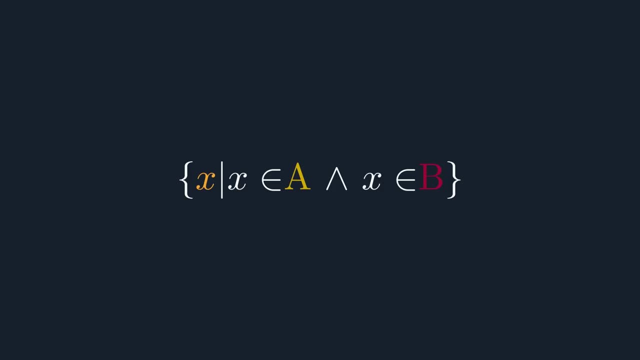 elements, and that is the fact that the set of elements has very short and undescriptive names everywhere. even if you may notice the naming scheme of using capital letters for sets, you may still ask yourself what X, a or B even mean. these are all variables that can basically be anything you want, so it's. 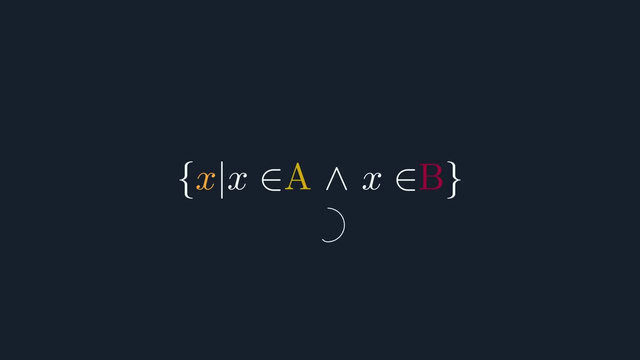 good practice to insert something into these definitions to make sense of them. for example, if you substitute the sets a and B is going to be orange. The reason I put so much emphasis earlier on the if and only if phrasing is that a lot of statements are merely just implications. 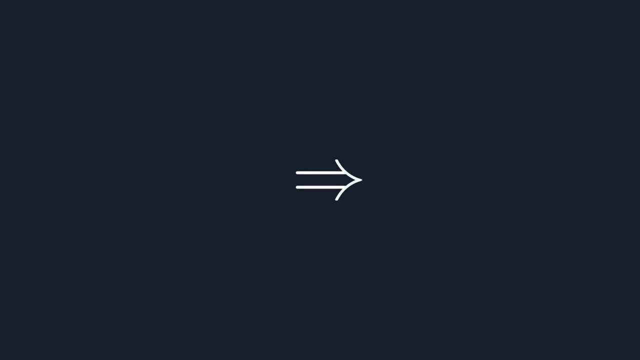 or conditionals, which are kind of similar but only work one way. They consist of two arguments, the first of which we will call the condition and the second the result. An example would be: if two natural numbers are odd, their sum is even. 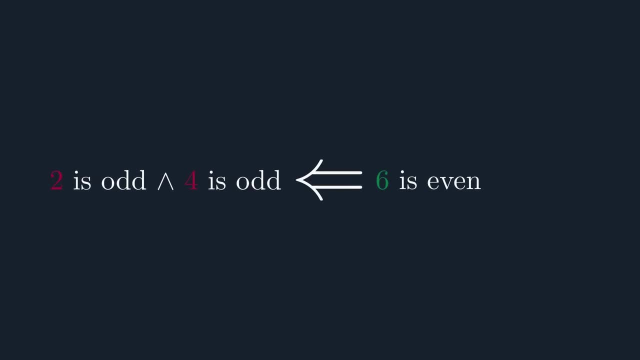 If we reverse this statement, it becomes false, with two and four being an easy counterexample. Also, something to note is that we don't care about even numbers when trying to check whether or not our statement is true. This may seem very obvious, but it's an important detail. 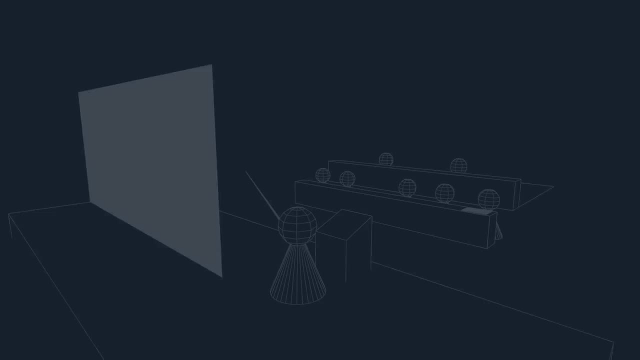 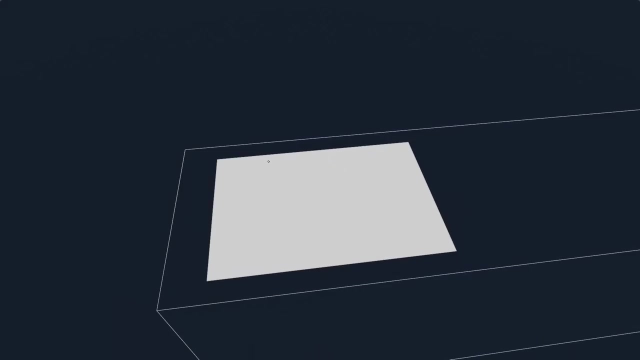 when approaching how to prove an implication. Let's analyze this last part with some information from earlier. The statement we used here actually concerns all of our statements. If we reverse this statement, it becomes false, with two and four being an easy counterexample. 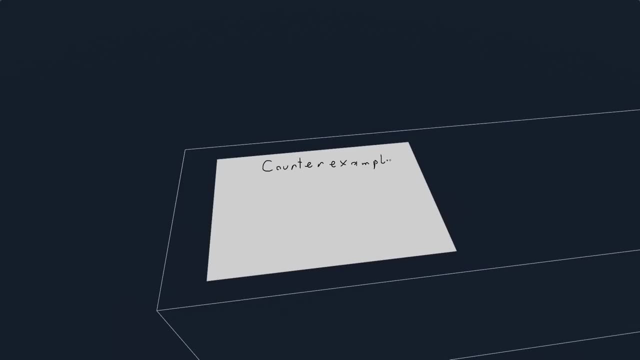 Which is why we could use a counterexample to disprove it, Using numbers like two and four to fulfill our condition of the sum being an even number, and then, using these numbers, we show that at least one of them, or in this case both, are not odd numbers. 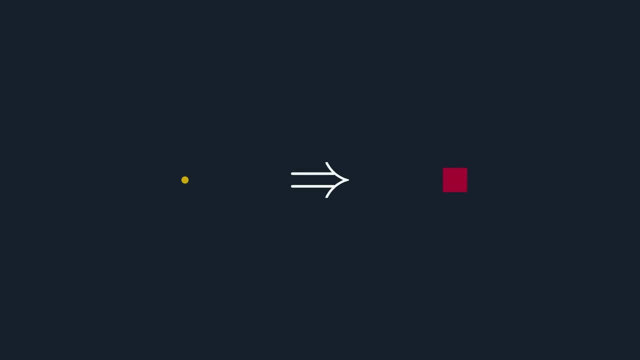 Proving an implication about all objects is a bit more tricky, but something any math student will have to do quite often, and it is therefore also quite important To do this. we need to assume the condition of an implication is true, namely that we have two numbers which are odd. 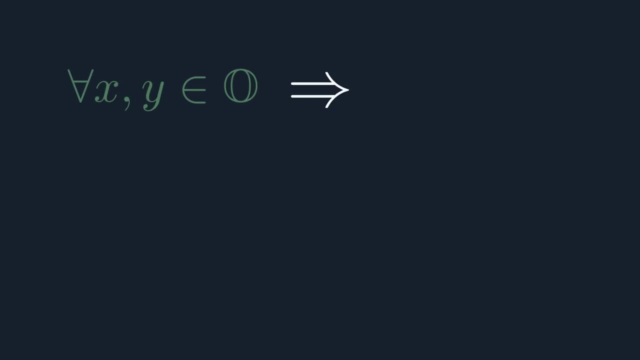 Let's just call them x and y and then prove the result, namely that their sum is even. To show this, we know that any odd number can be expressed by an even number plus one. So we can express x as x, even plus one, and y as y, even plus one. 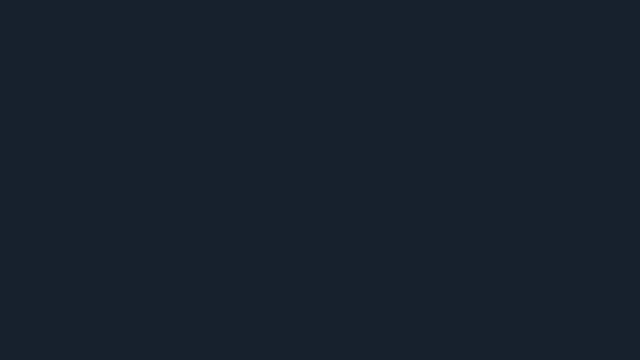 Again, if all these symbols or nondescript variables are confusing, you replace them with some meaningful substitutions, like 5 for x- meaning x even becomes 4, to make sense of everything. With this we can express the sum of x and y as a sum of two even numbers plus two. 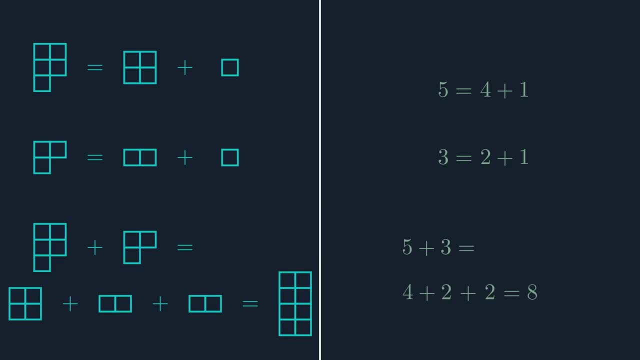 which is then even. This proof, of course, depends on the knowledge that the sum of two even numbers is even, but you will quickly understand why. So let's start. You will quickly notice that, in maths, any proof depends on some given knowledge before it. 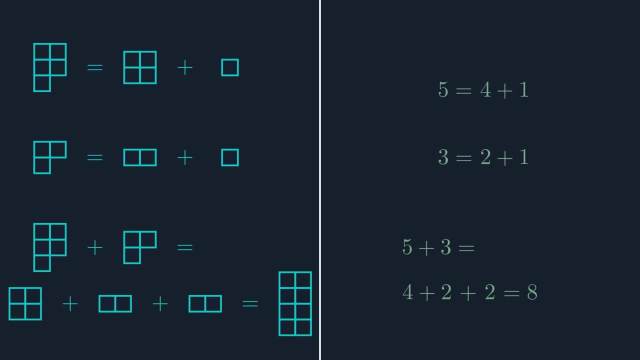 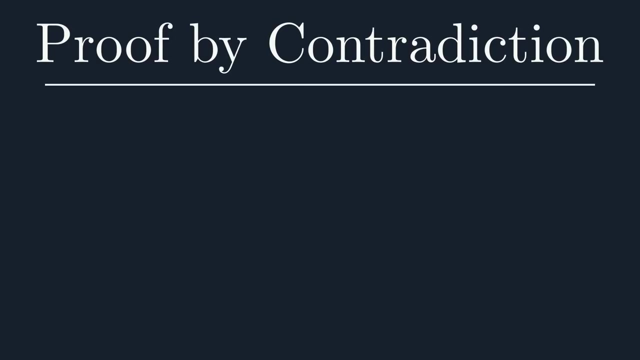 And at some point down the line you will just have to make assumptions about the existence of numbers. But that's a topic for another video. A neat trick when trying to prove an implication is something called proof by contradiction, which can often be easier than proving a statement directly. 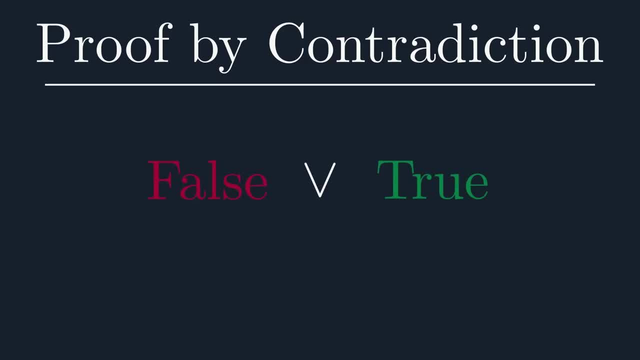 We know that either a statement or its negation must be true and an implication is false if, and only if, the result is false but the condition is true. We can use this knowledge and show that if the result is false, the condition must also be false. 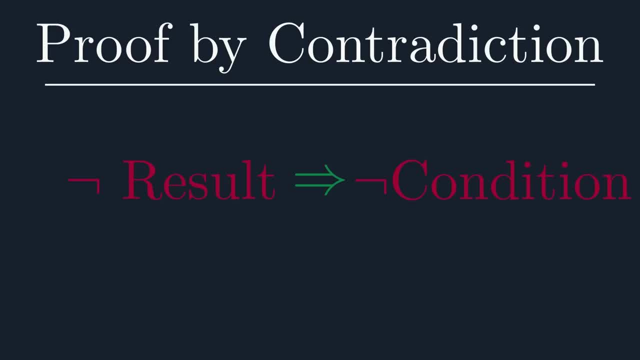 and from there we follow that the statement must be true. If you didn't quite get that, don't worry, it will be way easier with an example. Suppose we want to prove the following statement: Let's use n as our variable for a whole number. 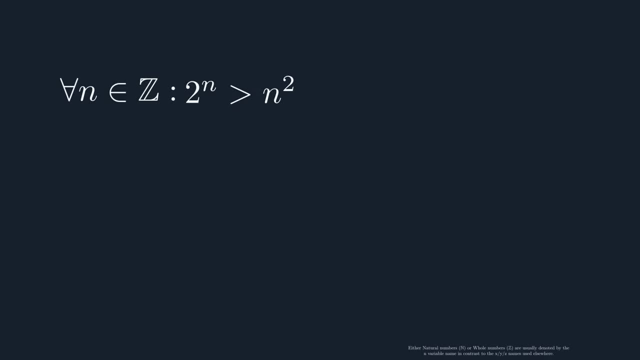 If 2 to the power of n is greater than n squared, then n is greater or equal than zero. To use the proof by contradiction method, we assume the negation of the implication, so n shall now be a negative number. If that is the case, then 2 to the power of n is a fraction. 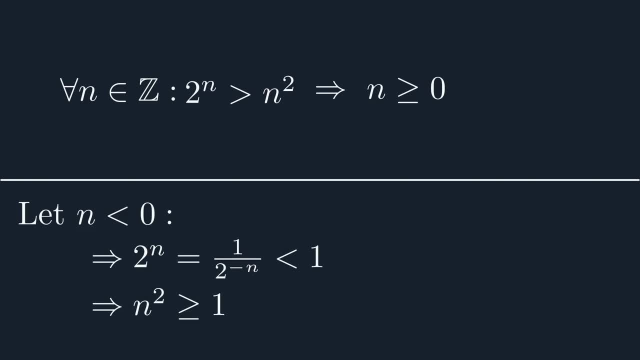 but n squared is still just a positive number, meaning 2 to the power of n is smaller than n squared, And since this is a direct contradiction to our condition, we have now proven that this is impossible and that the statement is therefore true. 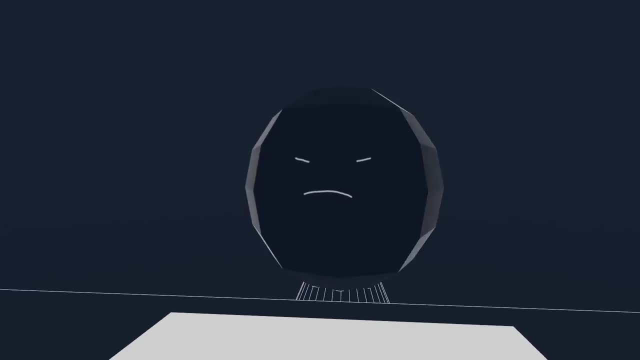 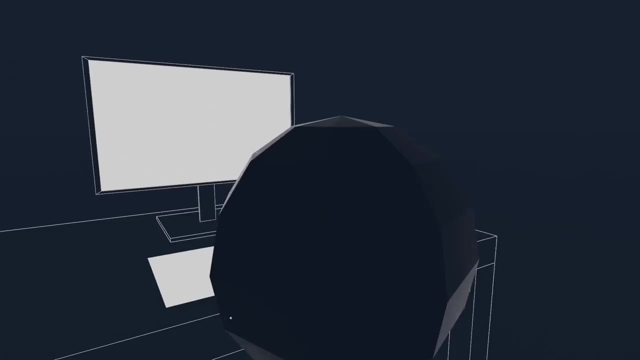 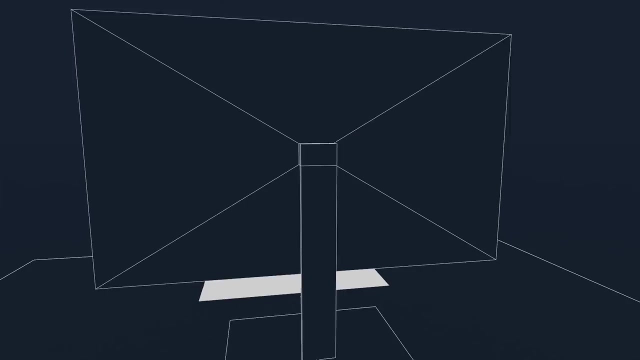 Now, if you are someone starting with your mathematics studies at university and you find yourself struggling with proving stuff for the exercises, I would recommend practicing formalizing logical statements, That is, taking natural language statements and writing them down using quantas- logical operators- so you have something concrete to work with afterwards. 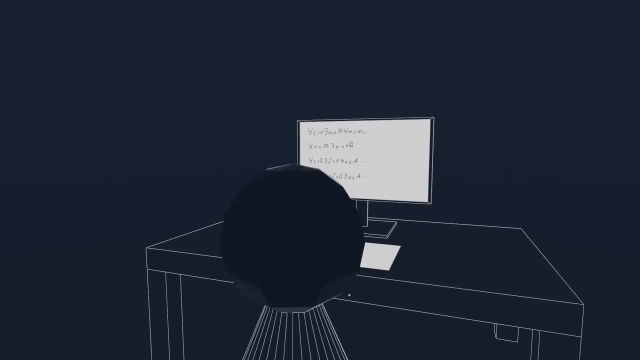 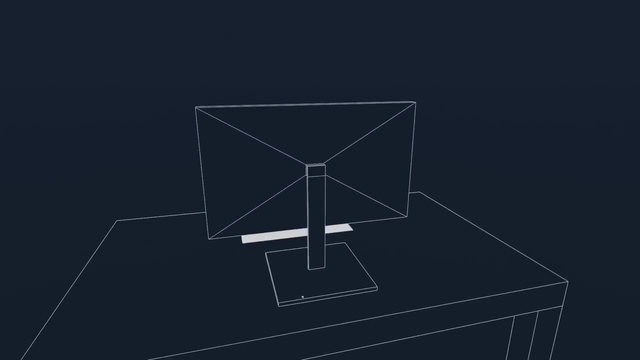 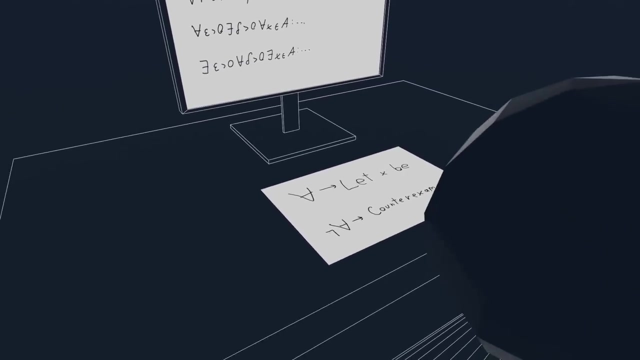 And once that's no longer an issue, make sure you have a methodical approach to solving those formal logical statements. If you have to prove something for all elements, don't be overwhelmed and just start with the methodical approach of choosing an arbitrary one. 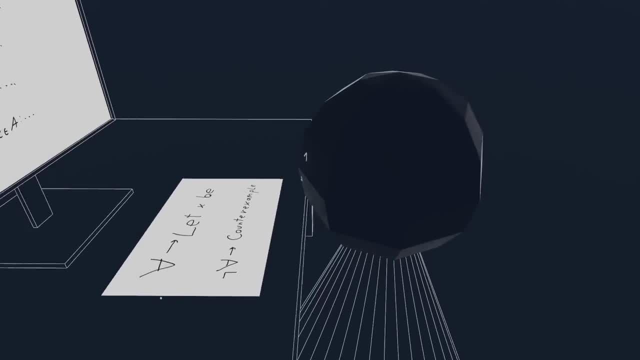 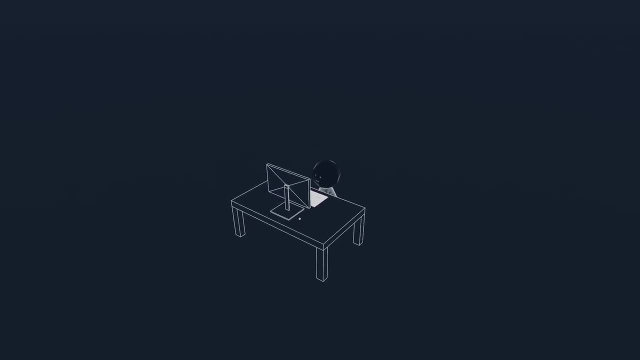 and think about its properties and what you can conclude from those. Even if a problem seems very unsolvable, approach it formally and then check the tools at your disposal. Alright, once again. thank you so much for watching. I'm not sure if this video will do too well, but I thought it's a very important topic that.